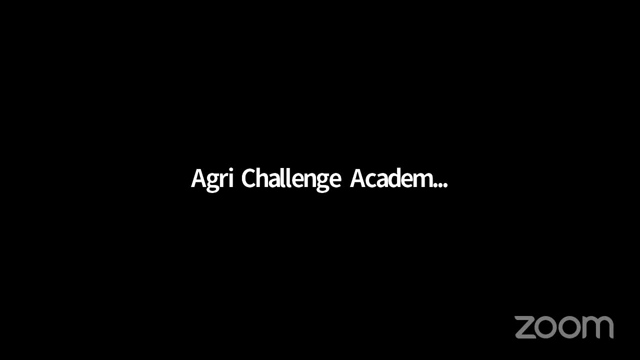 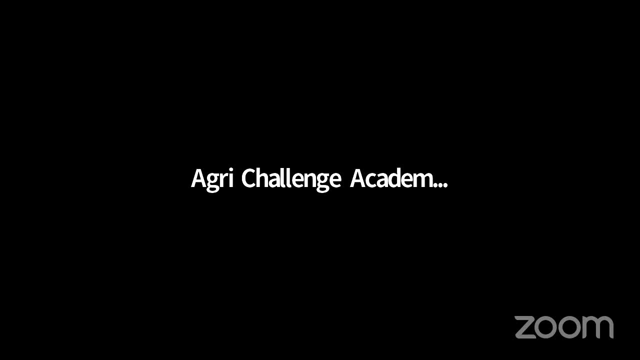 a lot of students again. okay, we will wait up to 2: 45, then i will start. you, you, you, you, you, okay, students, good afternoon, i think. uh, that's all the strength is for today. totally five students. where i came, hardly we can see a five student. 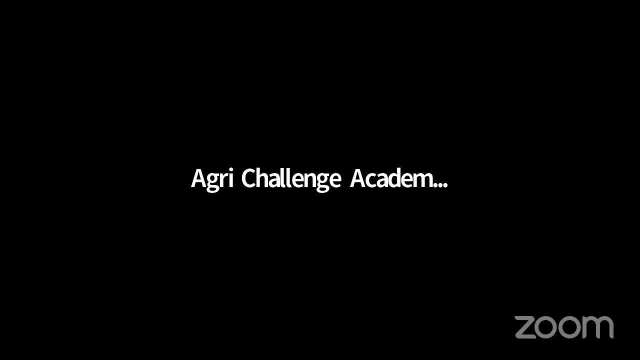 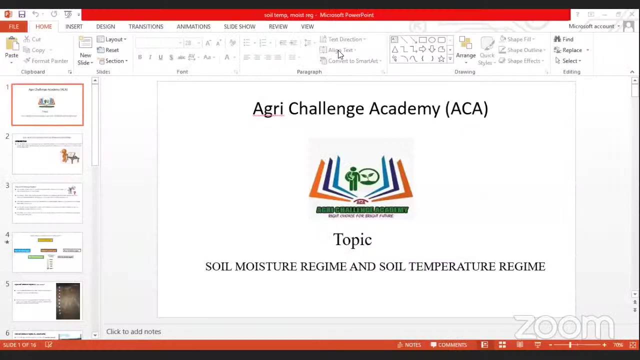 students. right, uh, very small lecture to students. very, very small lecture, but very interesting lecture. we will see what is done. now i will share my ppt, right? is it visible to everyone? is it visible? yes, okay, my voice is clear, right, uh, okay, thank you. uh, well, students, a very small lecture, but. 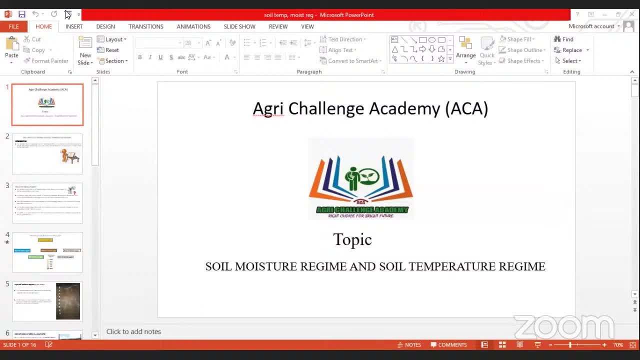 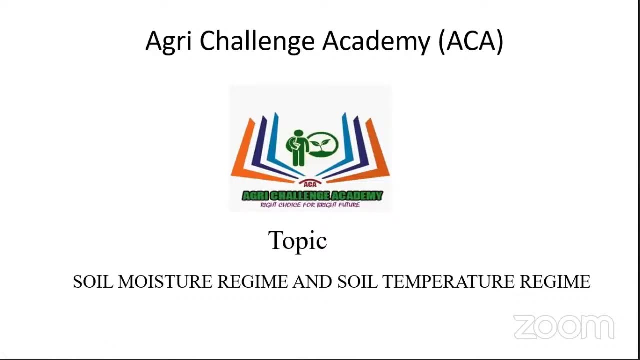 this lecture will play a important role in our pedagogy, pedagogy or pedagogical classifications, etc. i should, uh, i should mine in that and i will start my lecture. this is so. today's topic name is soil moisture regime and soil temperature regime. so, students, you remember, on the 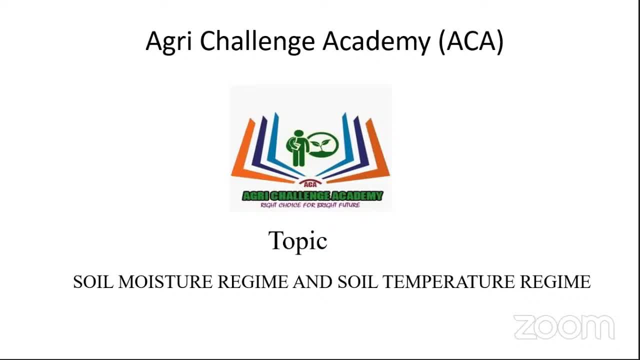 thing at very for a very starting of our pedagogy classes, we have learned about the: what are the important soil forming factors, those five soil forming factors, and later we have discussed about the. what are the different type of specific and important soil forming process, or phylogenic? 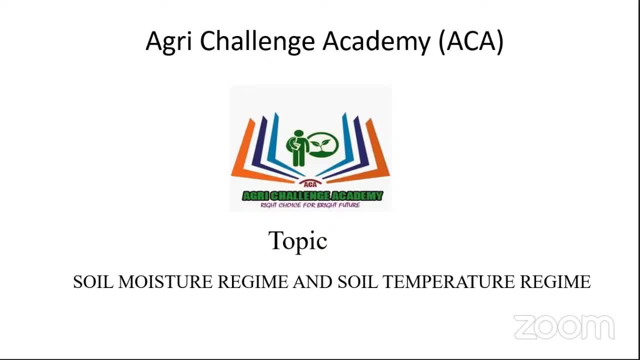 process, that elevation, elevation carbonate, this or calcification, lateralization, etc. etc. we have learned everything and after that we have learned many things. and now we are. we are end up here: soil, moisture and temperature. remember, students, moisture and temperature both place a major role in biologically both the micro microbial activity will completely depends upon the 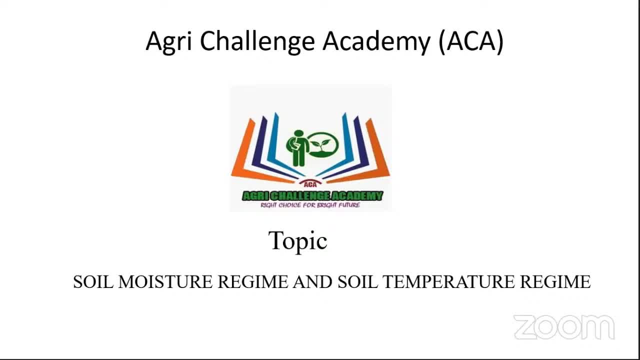 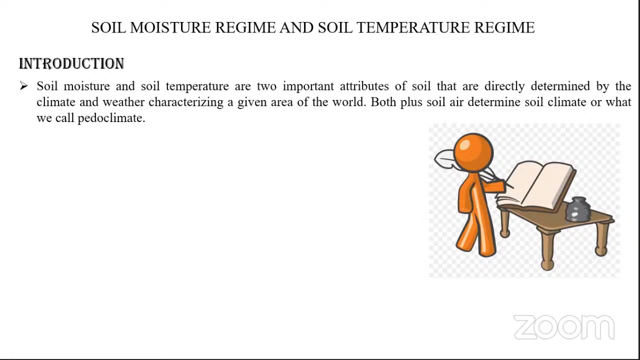 active importance of the moisture and temperature. so this- both soil and moisture regime also plays an important role in the soil development. that is pedagogical development also. now we will see what is an importance of soil moisture and soil temperature. regions- you very first, students introduction. so soil moisture and soil temperature, both are two attributes of soil that are directly 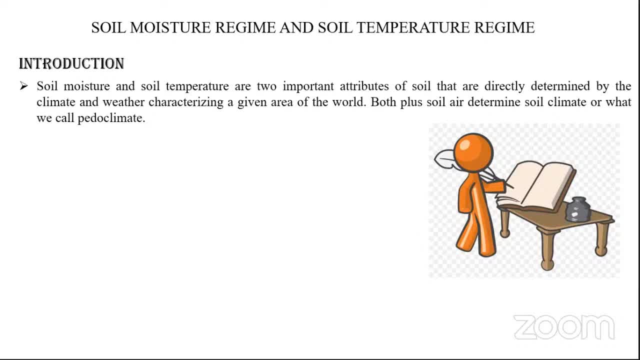 determined by the climate and weather characterization at a given area of the world. so, as i said in, as i said in the year, both this earlier, both this moisture and temperature plays a major role in weathering, or weathering, and completely determined by the climate and weather. 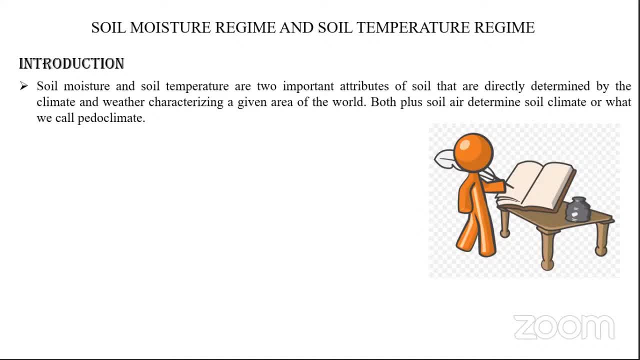 conditions, and this includes also soil air, soil air and soil climate and whatever called pseudo climate. what a pseudo climate means, students? it's not a real climate. it's one type of climate so which is completely depend upon the climatic conditions. right now we will see, one by one, where you need. 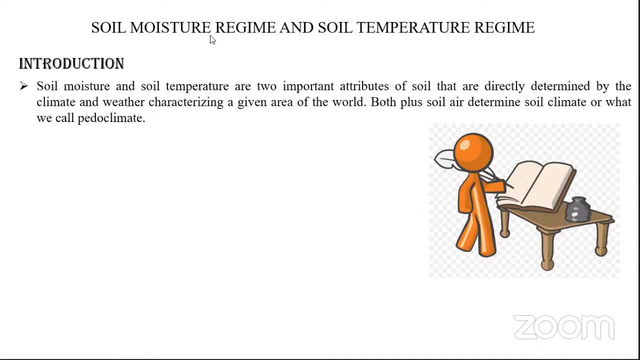 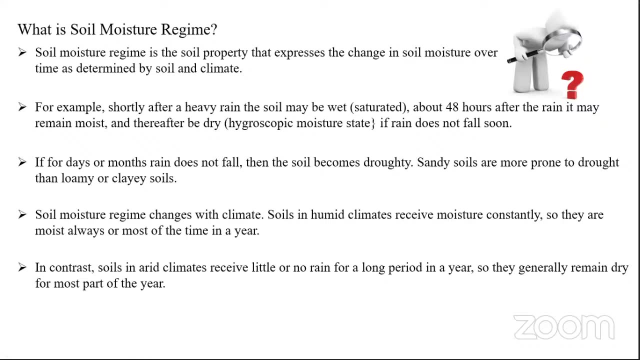 these two in. we will read these two in a one heading, okay, next, N, M, M, A, R, S, Q, P, S, T, A, V, S, W, C, Y, V, Y, Y. if it is completely, soil is completely saturated, completely, there's enough. what is there about 40? 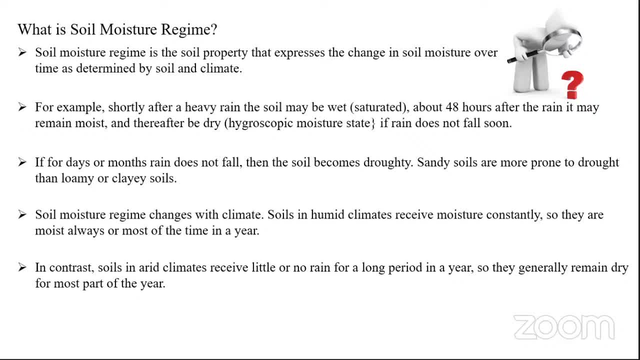 years. what do you? what do? what we say? it's completely saturation in condition. and about 48 hours after rain- i mean after operating- what will happen? the moisture will be drained, or some moisture will be drained out. it will be up to field capacity. you will have you all this learning. 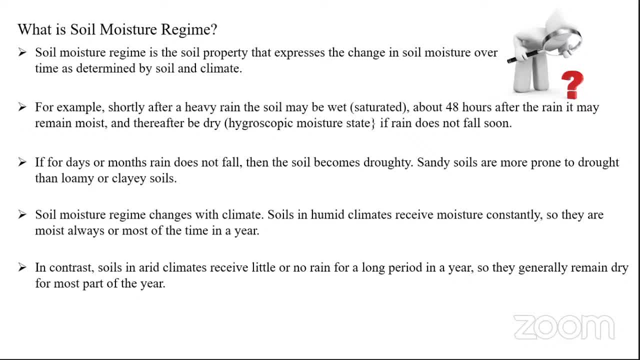 or irrigation algorithmic courses. that's called field capacity. thereafter, what will happen after completing complete drying of moisture? what do you say? there is a small amount of moisture, very little amount of moisture, that that state is called hydroscopic moisture state. this is what we will learn if the rain does not fall, if there is no rain, and whatever the enough moisture is. 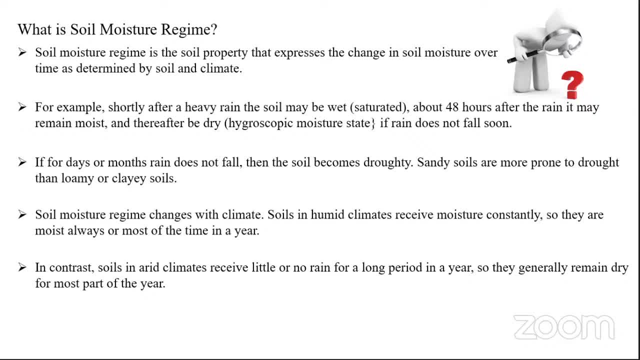 completely dried up due to the heavy summer or heavy hot temperatures or in arid conditions. what we say is due to the hydro. the laptop marsh is completely hygroscopic moisture state and also students. it takes for about the days and months does not fall. what will happen? the soil become. 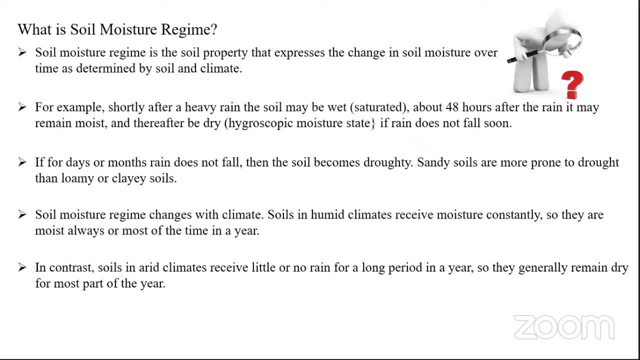 drought completely? there is no, you know, not at all. there is no rain. what we will say? that condition is called droughting condition. sandy cells are more prone to the drought than low missiles and clay cells. why? why, students, you should answer? sandy soils are more prone to the drought. sandy cells are very prone to the doubt when compared to loamy. 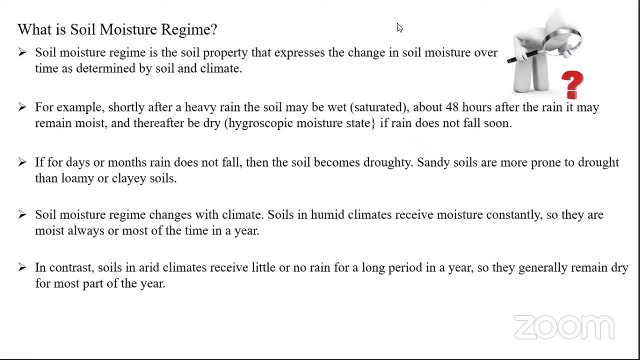 and clay soils. what is the reason? what's the reason? clay soils have more water holding capacity. yeah, more water. clay, clay and loamy soils have proper water holding capacity and also physical conditions. chemical conditions are very, very favor in in this in case of loamy and clay soils in the in. 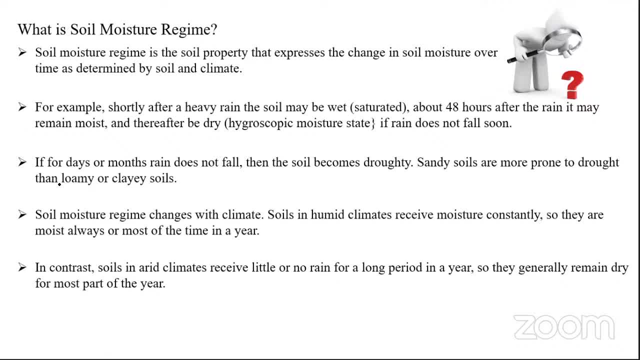 loamy and clay cells here, loamy and clay. in these, these two conditions, we can see loam and clay, whereas in sandy cells with very poor structure, what will happen? whatever the robot or the moisture you give, completely drained off. there is moisture holding capacity very, very little okay. 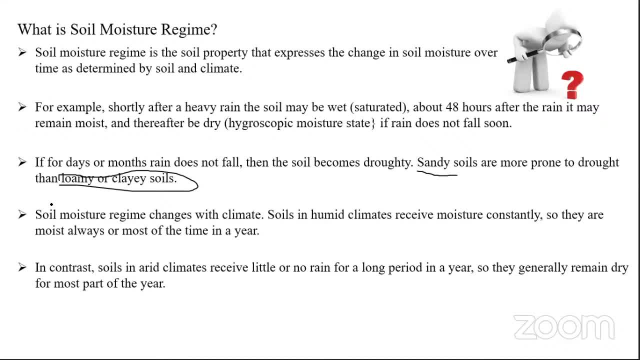 and coming to current wise, this is almost all wanted and i think then we still have to look at how we can of lesbian and lesbian girls in western. okay, so hope that we could take some more a wore back. so with the climate, so, for example, if it is a humid climate, resource moisture constantly, if there is. 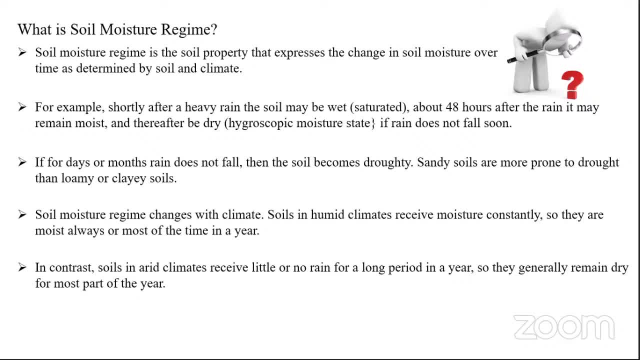 like the, if the climatic conditions was completely humid conditions, very, very enough precipitation is there. what do you say? there will be complete. there is a continuous receiver of the moisture. so they are called: they're moist always and moist twice in a year, mostly this type of conditions. 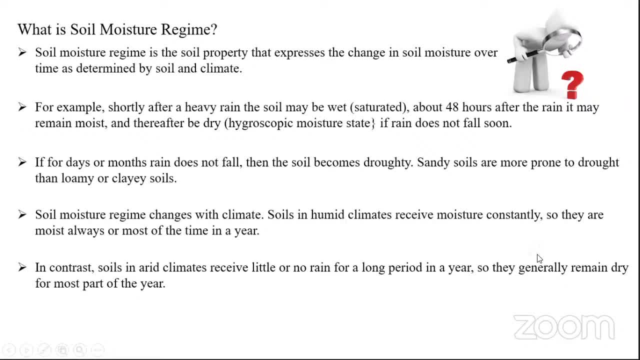 especially. you can see this type of humidity, this type of complete saturated moisture conditions. you can see in a where the humid conditions are, in contrast, in reverse, opposite to what we said. if there is a soil, certain arid climate, you receive very little, have no rainfall for a 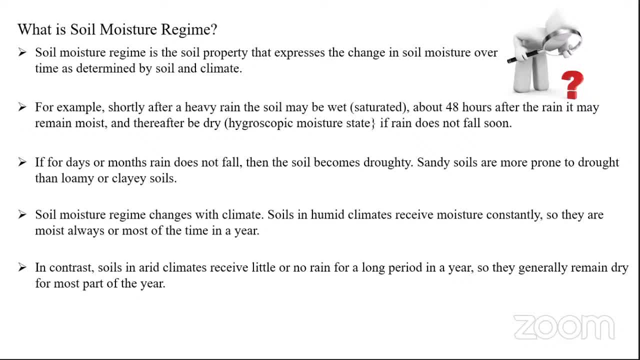 longer period. so generally that remains dry from most of the parts. so this is the thumb rule, students. if it is a completely humid region, we can see complete moisture, moisture conditions. the moisture will be very more in humid climate conditions directly opposite to another section that is called the arid climate- arid area area. it means it's complete. there is no precipitation. 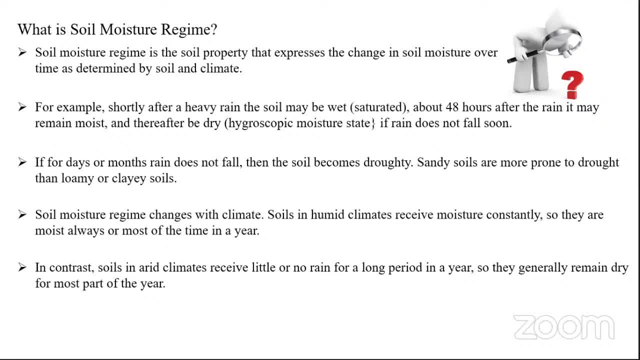 no precipitation is no rainfall, so naturally it will become a uh, very dry and complete. most of the parts of the year, this is called completely dry conditions will be there. so you remember these, these thumb rules, and also remember this point also. so, based on based on these three ideas, we are going to study the soil moisture region and also you will see, 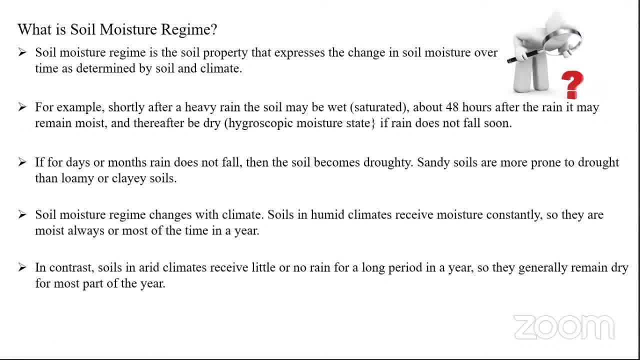 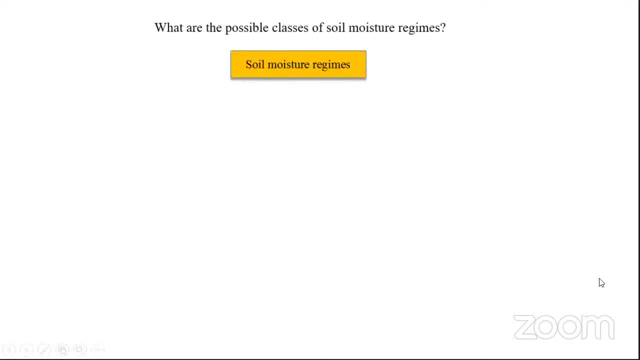 some different terminologies. those terminologies are very, very important for your competitive examinations. we'll see next. so what are the possibilities? what are the? what are the possible classes for the soil moisture region? so how many times? what are the possible classes means how many possibilities. how many types of soil moisture regimes are there? 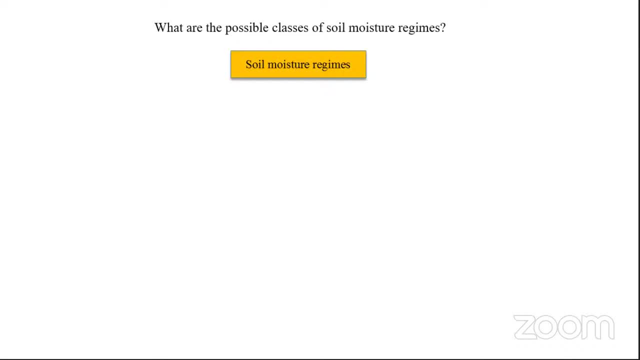 we will see. what are the regimes. what are these? very first one: please note down these terminologies please. in soil science, the terminologies are very important. you will get most of the questions from these terminologies and their values. typical values will be there. those values are important. 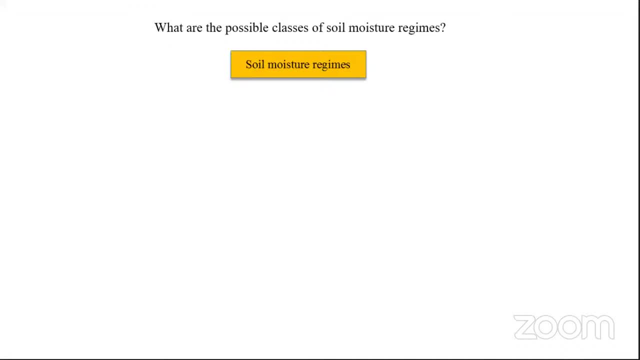 to us. only from these values, only you'll get most of the questions. very first one, very first one: students, a quick soil moisture regime, active, active, full of saturation. you will read. you will read all these things about incoming slides. first, we dictate soil moisture regime, crafts eye and moisture regime, eritic soil moisture regime. 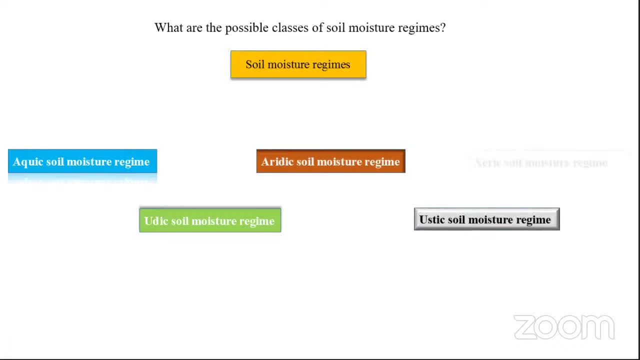 district soil moisture regime. xeric soil moisture resin. so, naturally, these are the different types of any soil moisture beauty. so, sigmarodux, these five types of soil moisture regimes are present at present. we will read, we will see. we will read the soil moisture regime under these five headings. so these five words, or these five, 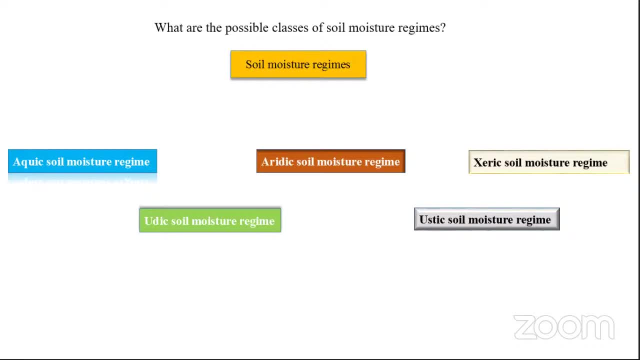 headings are very important regarding this lecture. so remember these five lectures, these five words, and you will. you will get many questions, students especially- uh, most of the questions. if you go to the central fertilizers you see co or record some triandrum chemicals. there are many, is there? 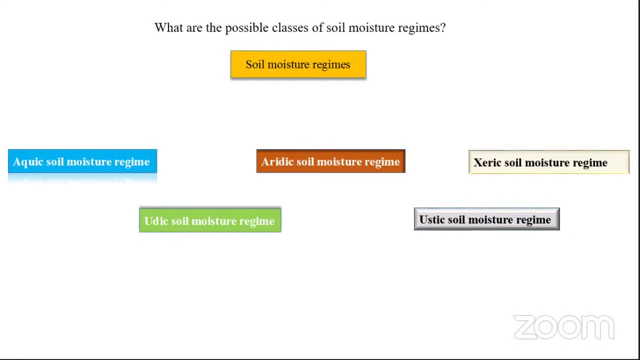 not fertilizer companies. they will. they may, i mean in my interview. they may not ask, they may ask in your examination. so naturally, students just just note down this one: if you are not taking, take note down, if arid is very arid, ziric stick udic aquic. it means if you are going, coming down. 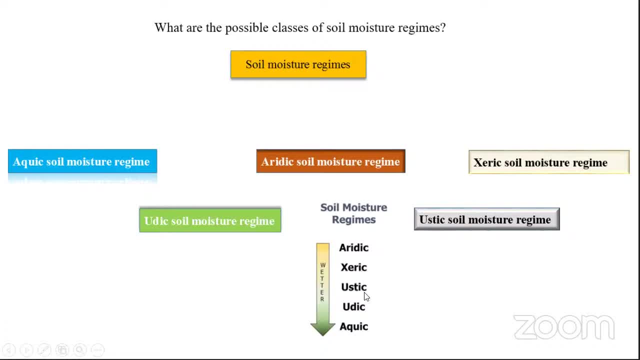 and down. what will happen? arid. arid is very dry, ziric is somewhat dry, somewhat wetting. stick is somewhat wet, udic is moderately wetter. come to aquic means completely saturated you. that's why, if you're going down, that's my vector. i mentioned here vector. so if you go to the array, 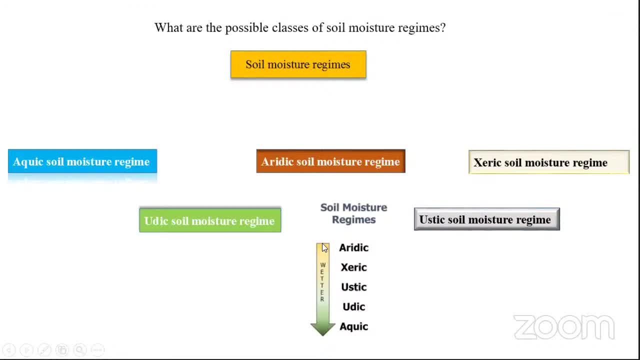 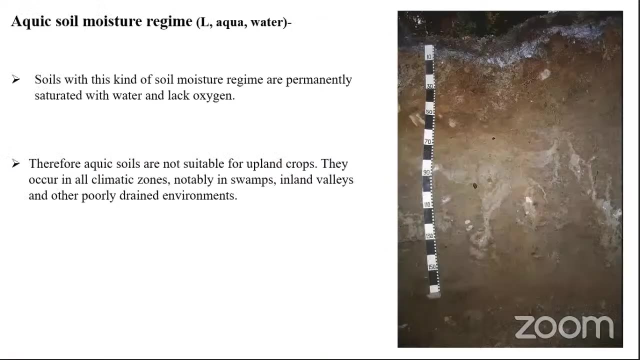 array, erratic, ziric, the stick, the dick, active. if it comes down, it's complete. there will be complete. moisture will be increased like this. please note down this to us, please note down, be careful. okay, very first one, a quick soil moisture regime. l? l means latin word strength, aqua means 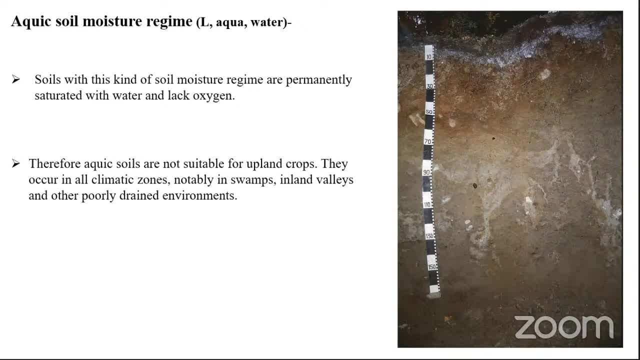 water. sorry, l means some scientist name, i think, so i'm not sure i want to inquire. aqua or water, aqua equity, aqua water, so naturally we have a one brand also in water. water based aqua phenol is water. aquic. soil moisture regime means soil with this kind of soil moisture regime are permanently. 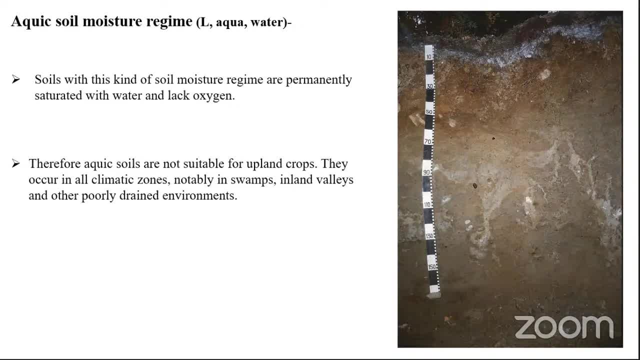 saturated with water and lack of oxygen. so naturally, what will happen is permanently they are completely saturated with water. and what will happen? there will be no oxygen. there is no supply of oxygen, so completely anaerobic conditions will be prevailed here. therefore, aqua soils are not. 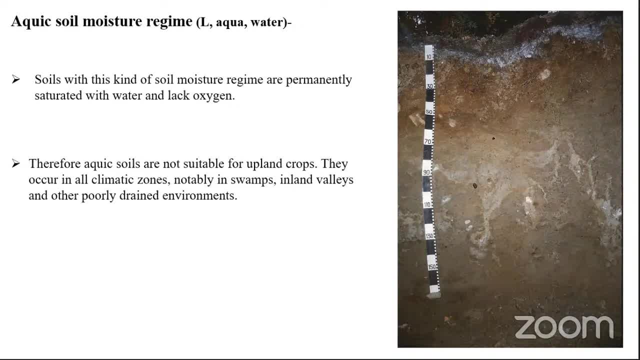 suitable for the upland crops. they occur in all climatic zones notable in swabs and inland valleys and other poor drain environment. environmental, mostly in valleys and more in some some poor drainage conditions conditions you can see this type of soil moisture regime, this type of active. 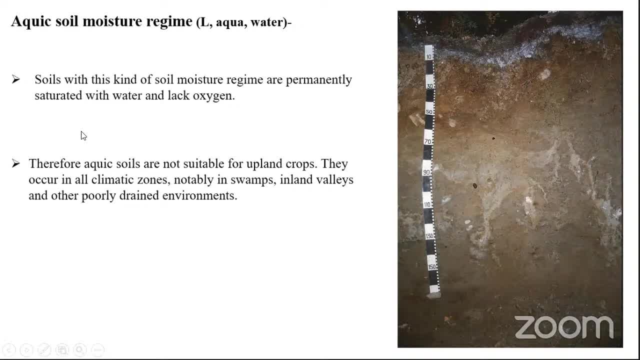 soil moisture regime. you can see in, in such type of conditions, inland values and swamps and other other poor food rain conditions conditions. we can see aqua also. this is the. this is the conditions in aqua soil moisture regime. remember, students, aquic means water. this here in this, in this type of marshallism, completely. 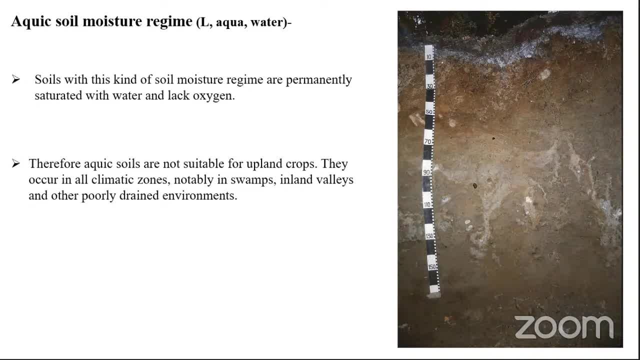 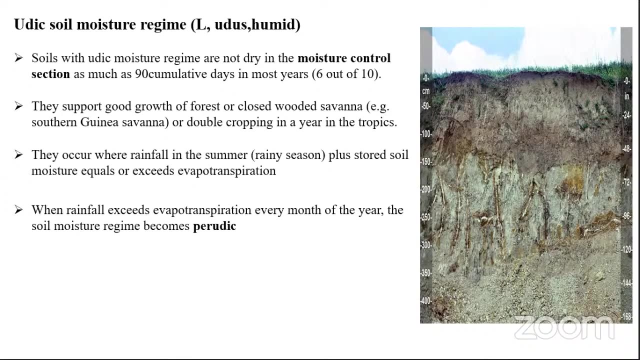 there will be a saturation of water and lack of oxygen. we can see in this type of condition- this is regarding with aqua soil. i mean to that eudic soil. marshallism means humid, you make humidity. it's complete. remember, students, as i shown in that image. 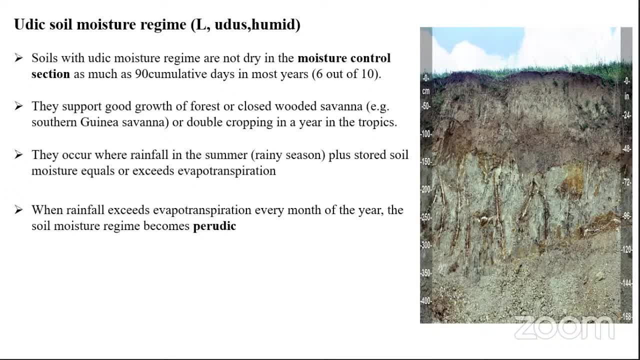 as a in a reverse model, but i'm teaching in another model, so try to identify it okay. eudic means soils with edict moisture regime are not drying more in the moist control section as much of 90 cumulative days in most of the years out of six. or i mean some particular area, not 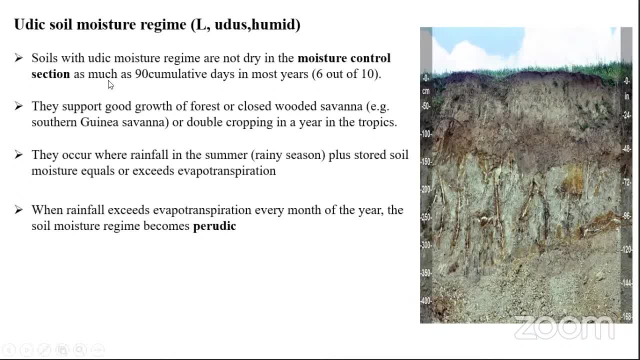 entire areas may not be dry. students and some particular sections will be in completely moisture in a 90 continuous days- 90, 90 cumulative days- there will be completely saturation. they support good growth, naturally this type of uh soil marshallism. they support good growth of forest and closed wooden savannah. savannah means 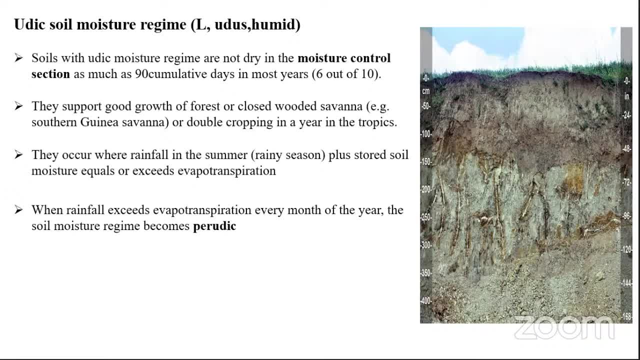 geneva you can see some savannah forest is there now. you can see this type of conditions, a double cropping in this area, in this topic. naturally, if this type of soil martial condition is there, we can go for the double cropping in here. they occur where rainfall in summer. 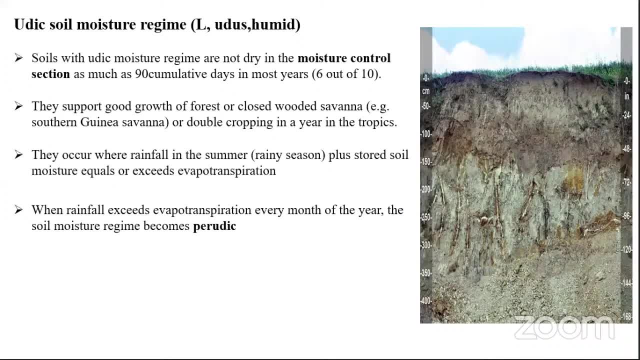 less stored soil moisture equals or exceeds the vapor transformation. naturally, students, um, naturally they occur when rainfall in summer. i mean they they some unseasonal rainfalls or some in some rainfall in summer season, plus plus in moisture, and when the moisture is exceeded than the evapotranspiration, we can see this type of conditions okay when rainfall exits evapotranspiration. 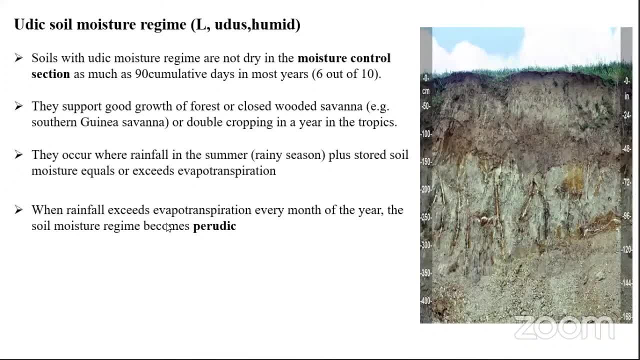 every month of year, the soil regime becomes pre-edict. actually the condition is like this: when the enough moisture condition is there and vapor transpiration for every month or often year, pre-edict, soil moisture region edict and periodic if the evapotranspiration makes it means this. 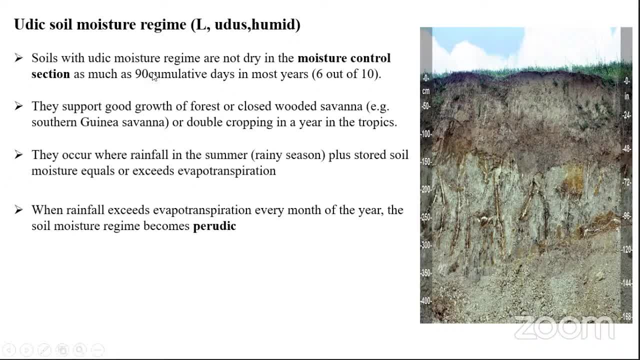 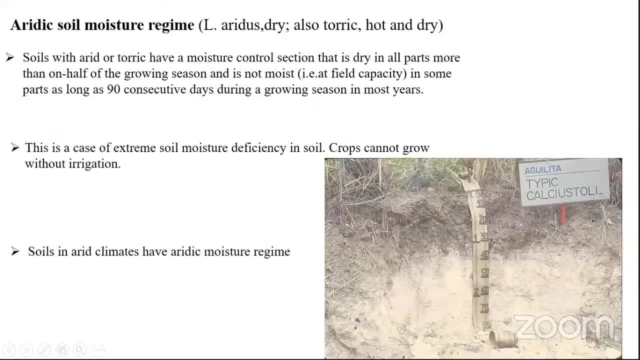 called the pre-edict conditions. this is: this is regarding with the edict, soil moisture resin and another one is erratic soil moisture and it is dry, also toric or hot end. naturally, aridus means dry. okay, soils with arid or toric have a moisture control section that 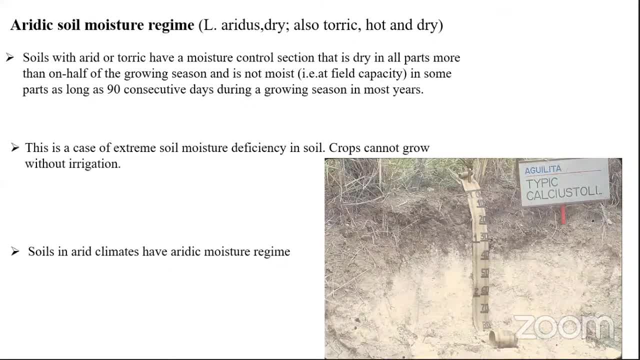 is dry in all parts more than more than on half of growing season and its moisture mostly design and parts most 90 consecutive days completely. there is no moisture here is available. respiration is very less, continuously 90 days there there will be more. the soil will completely will be dry. 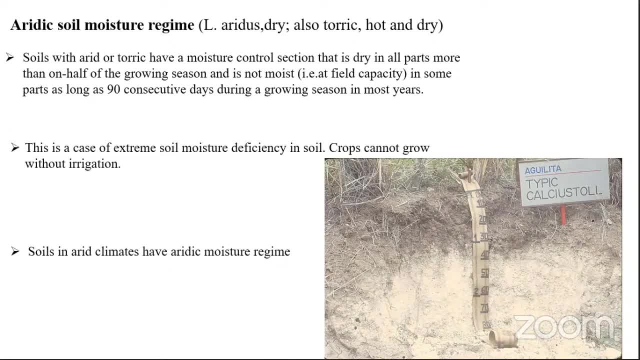 conditions, dry conditions, and this case is extremely soil moisture deficit in the soil and crops cannot be grown without irrigation. if the condition is like this, if the soil moisture is in this condition, erratic soil moisture moisture regime means what will happen: crops cannot be grown. crops cannot be grown without giving any example. so naturally, soils in arid 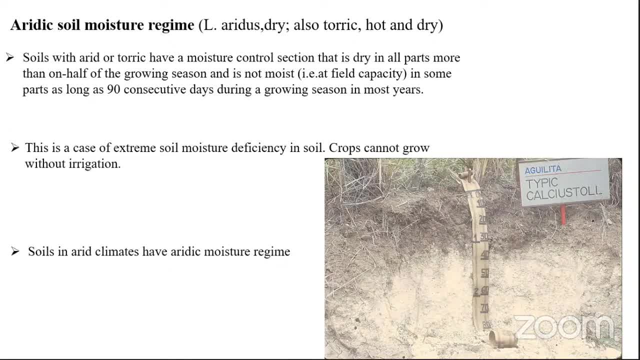 climate and climates, having have a erratic moisture regime, soils and arid climates. that means you will see these all these things in your further coming classes, students. in taxonomy you will see one order called erratic soils. in the erratic soils mostly you can see this erratic moisture regime because in lack of precipitation or lack of rainfall you can see 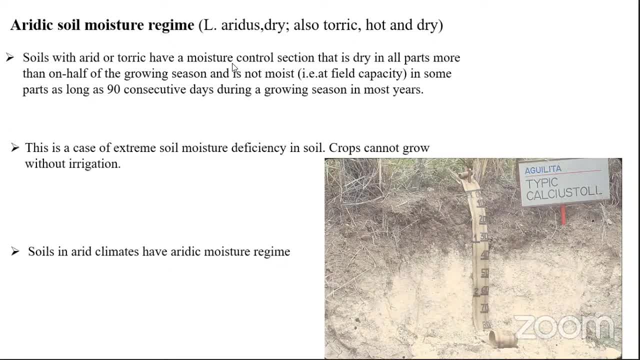 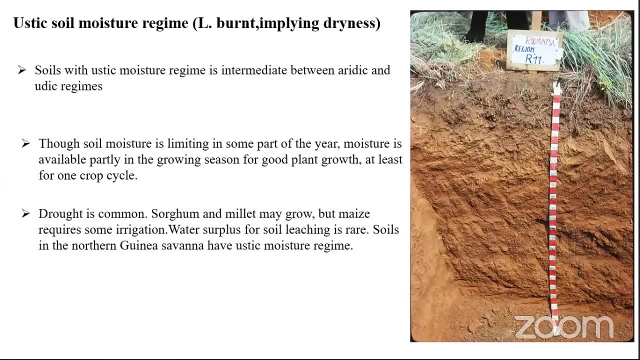 this type of soil moisture is next students, stick soil marshes and burnt or implying dryness. so it is somewhat. it is not neither dry not born. the soil with this stick moisture regime is intermediate between the erratic and the stick regime. as i said, neither dry, neither completely moisture. 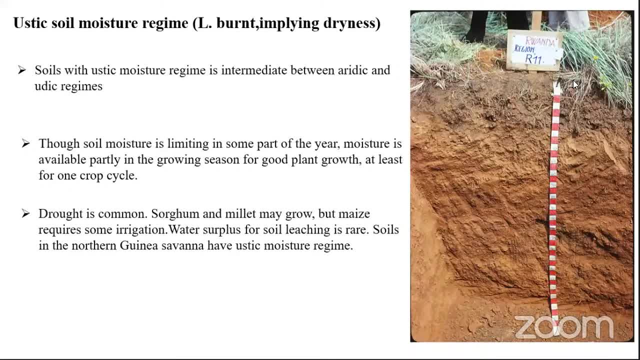 it is completely different. it is completely different though. the soil moisture is limiting in some parts of here. moisture is available partly in growing systems in certain areas. be very good plant growth at least. so one crop cycle, actually student, in this type of condition. it is intermediate storage, intermitted between the erratic and artists, so we can. 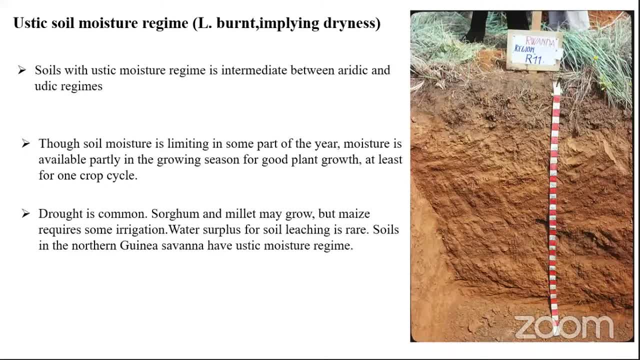 see some sort of moisture here we can say some part of good we can. we can go for one out one round trapping. that is one crop cycle. drought is common here, so we can see some drop draft very common. what are the different types of crops we can grow in this type of soil or stick soil? master. 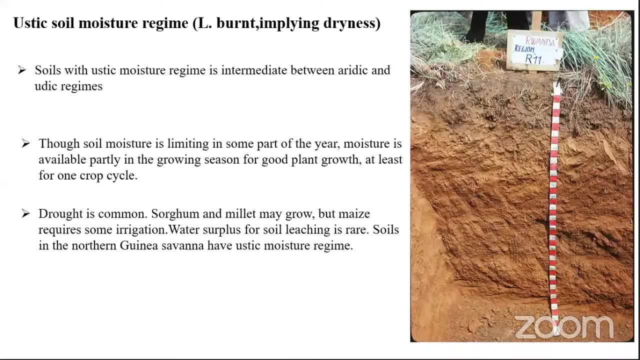 agent. we can go for sorghum, some sort of dry millet. naturally, what we, what we last, we have to be honest. so the our science silage and we are going to have macam. we have a lot of there space in it. rather, we have not identified any problem with the Weekly celebrating and 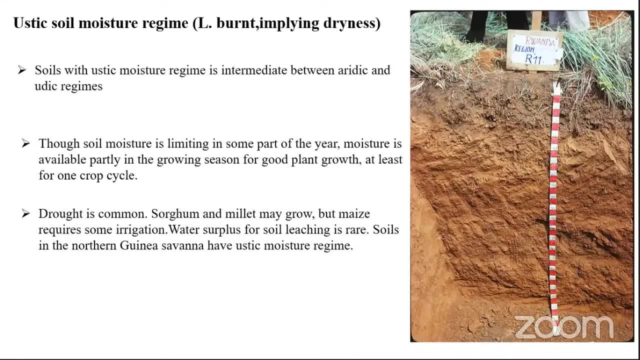 mestother. so we have to think what extract it is. so, for example, earth shortly already, plantation on a …. we have to filter out ships, laces and again soil moisture issues in soil moisture be grown. in our semi-arid zones we've grown other type of crops. we can grow in this time because 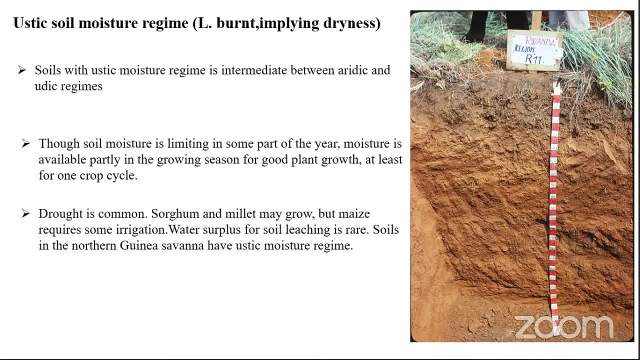 the moisture is very limited but maize requires some irrigation where water surplus for soil leaching is raised soil in northern geneva sam is mostly this type of this. actually is a some african nation. you can see where you can. you can see this stick stick moisture region. 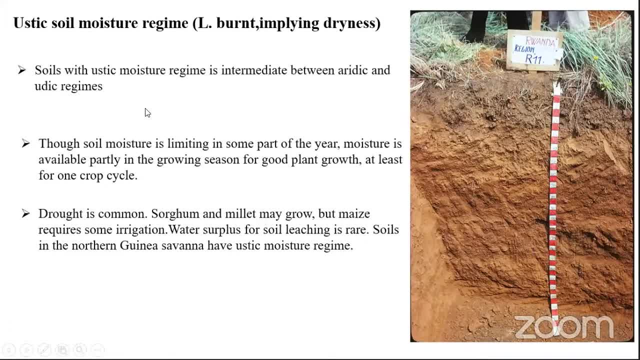 so sorghum and millets we can grow so naturally, students, here the moisture is very limited, but it is intermediate between the erratic and stick. your stick is intermediate between the erratic and the stick regime. so, regarding the, regarding the stick, soil moisture regime is this is: 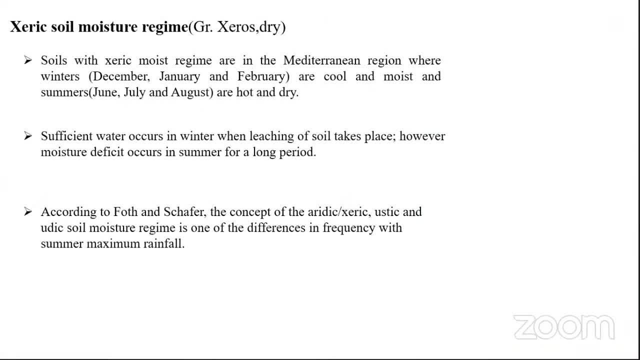 next xeric xeric soil moisture regime students, so soil with xeric moisture regime are in most, and military and region students mostly where winters materialism means it. here you can see students very cool, cool and moist. winters are very cool and moisture. summers are hot and rain. 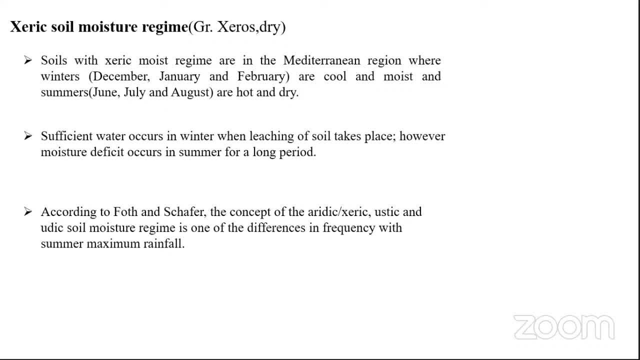 actually this type of conditions we can see, especially if you have anybody have a watching this uh, special geography or some animal climate channels, this type of play. they will show the mediterranean climate region. what are they? what are the soil conditions? are there, what are the animal or what are the crops? 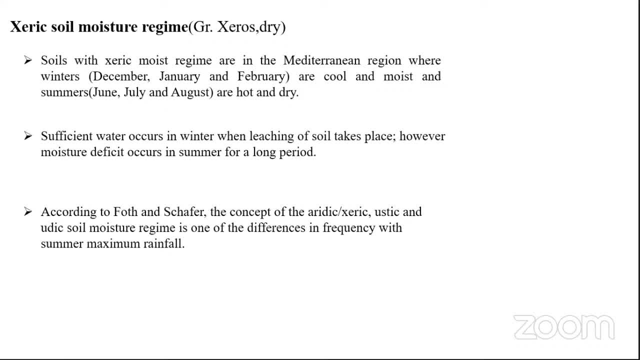 they are growing. we can see mostly material income. it is prevailed mostly in december, january and february. you can see winters. they're very cool and moist and at the same time in river summers- in zunzula and august- are very hot and red. sufficient water occurs in winter, naturally. 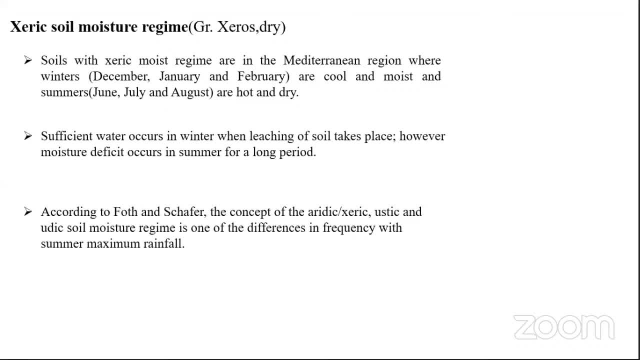 there is a cool moisture will occur in winter when leeches soil takes place. however, marsh deficit occurs in summer for a longer period. but due to the what will happen, due to the summer, there is no moisture. so naturally, there is no deficit of my dipshit of uh a moisture in summer, according to the food and stuff these two. 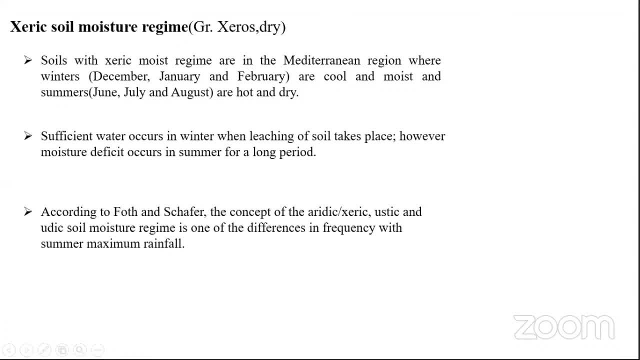 scientists what they're saying. the concept of erratic xeric stick and unique soil mushroom is one of the maximum rainfall they say. actually they have, given this technology these two is erratic or xeric. mystic analytic soil marsh is one of the difference in frequency of summer, in maximum. so in summer that's. that depends upon what. 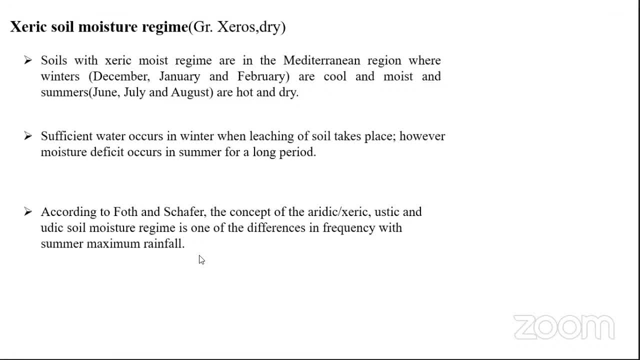 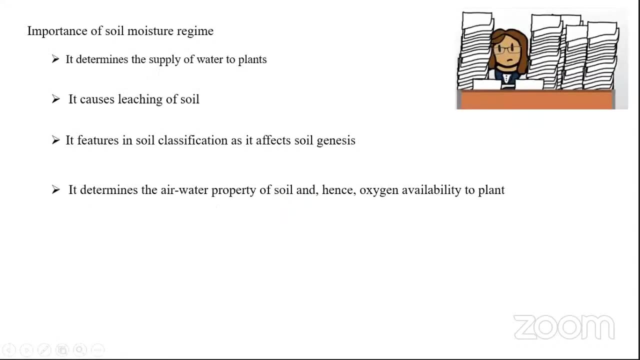 okay, let me repeat, okay. i think my signal is weak. that's why the voice is not clear about the, so naturally, the frequencies. this is what they both have said. next, so what is the importance of soil moisture regime? so why we are reading this much, why we have to read soil moisture regions, very first points. again, it determines. 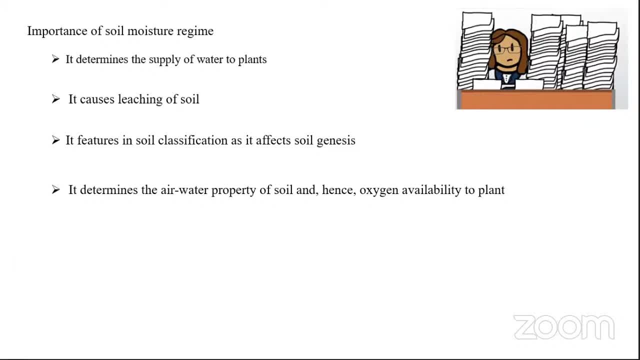 the supply of water to the plants. naturally, students, based on this soil moisture regime, it we can classify what, what is the supply of water to the water, or we can say what kind of crops we can we should grow to that particular soil. in case of leaching of soils, what, why it is. 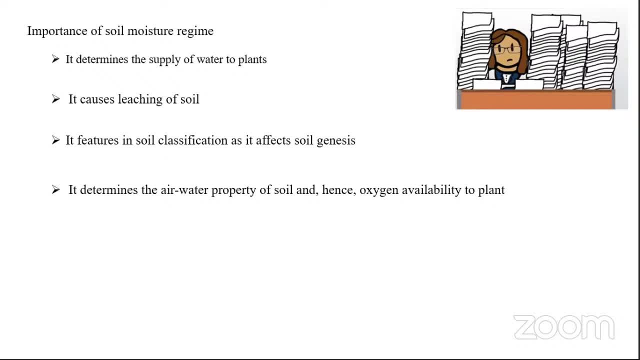 the cause of leaching on. what is the condition of leaching of soils. it futures in soil classification as it affects the soil genesis. naturally it will affect the soil genesis with the development of soil completely. the moisture will be affected. it will determine the air water property of 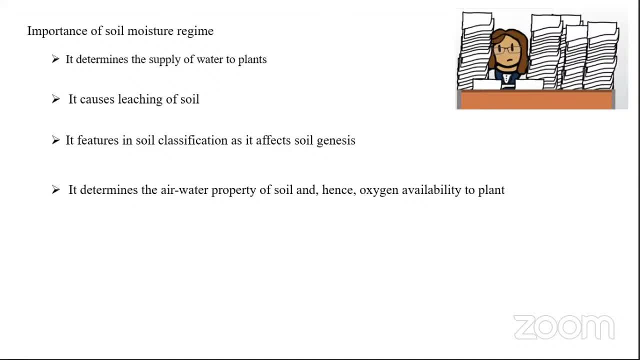 soil and hence oxygen ability of the plant, and actually the soil moisture, moisture. what will happen? the presence of air, our presence of the fox, is completely determined by the soil, the soil master region. so these are the four most important uh points regarding the soil moisture regime. so, regarding soil moistureism, this is it. if you have any electron, we will go. 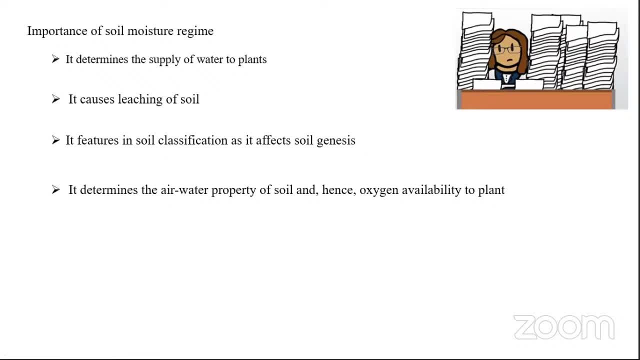 for soil temperature regime. you have any doubts regarding, uh, soil moisture regime? students, no, sir, okay, but be careful. this, uh, i think you are all from a bsc. finally, students, uh, please once read twice or try to understand once you go. once you get the grip on the soil moisture, soil temperature, the exam will be very interesting, okay. 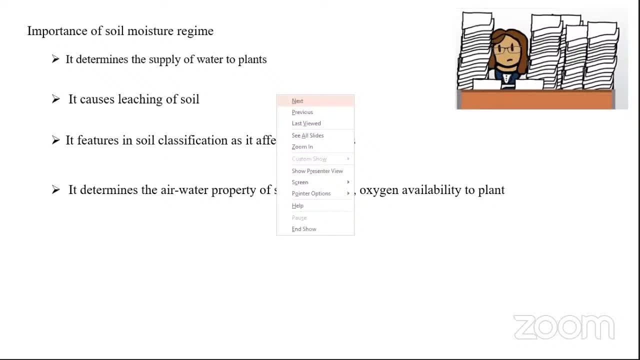 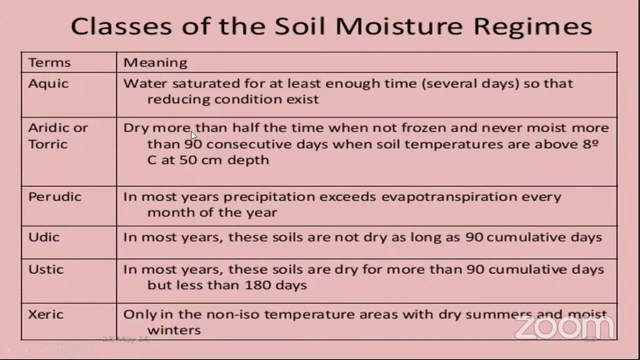 please see next slide. ah, this is today. actually, these are. this is my understanding. just for comparing. what i said is completely its easier. this is for your preparations: preparation. select this next: yes, the soil temperature is what is. the temperature also plays a major role in the soil week. 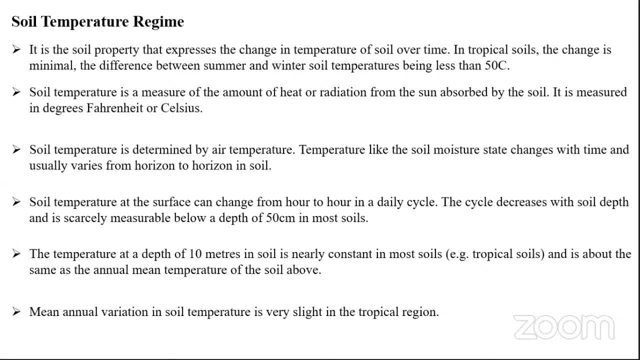 students. naturally, in soil it is a very, very fast. we will see the definition, students. it is the soil property that expresses the change in temperature of soil over a time. naturally, it will completely determine the temperature to complete the calculation or completely express, completely identifying or observing the temperature in over a time. in tropical size the change is minimum. 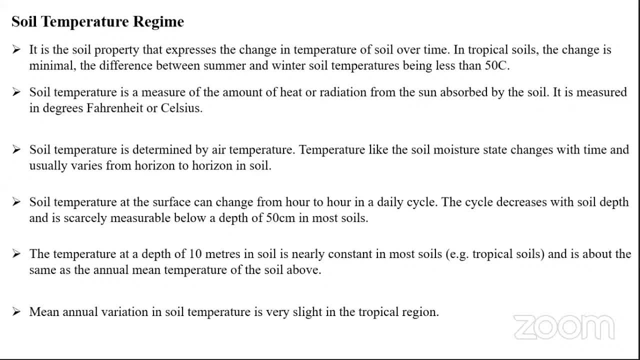 minimal, the difference between the summer and winter soil temperature being less than 50 degrees celsius. naturally, in tropical conditions where there is heavy summers, are there where we can, there we can see some. the temperature difference between summer and winter is very less. soil temperature is measured is the measure of amount of heat or radiation from the sun observed by the 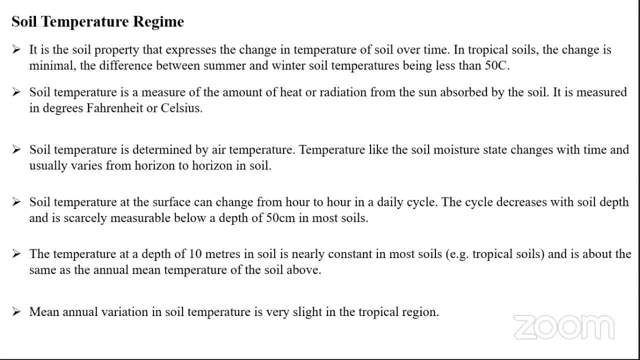 side. it measures in degrees of current heat or celsius. naturally, soil temperature is complete. it is a measure of radiation or heat from the soil will express in parent heat or celsius, uh soil temp and another what. my third point is saying that this temperature is determined by 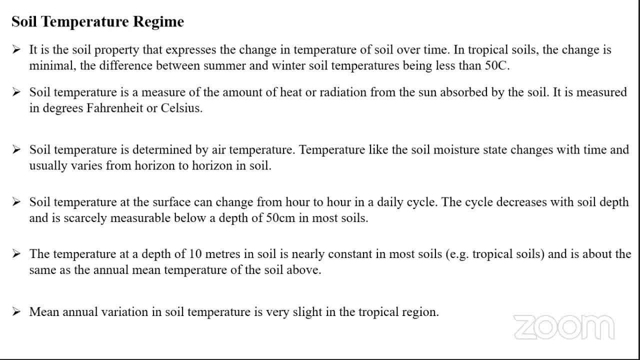 the air temperature and also it compared temperature. also soil moisture state with time and usually varies from horizontal and naturally the soil temperature is completely varies from horizontal, very, very topmost layer, maybe somewhat somewhat. there will be every temperature in daytime or sometimes in evening times. it will be less at the same time in evening if you go to the department layers. 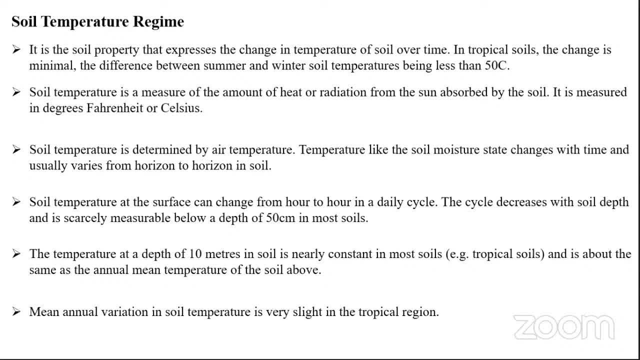 we can see. we can see that type of fluctuations in temperature in different different layers. soil temperature at the surface can changes from hour to hour in daily cycles. as i said, in morning it will be one type of temperature, evening it will be one type of temperature. in the end of most layers the cycle decreases with the soil, soil depth and it. 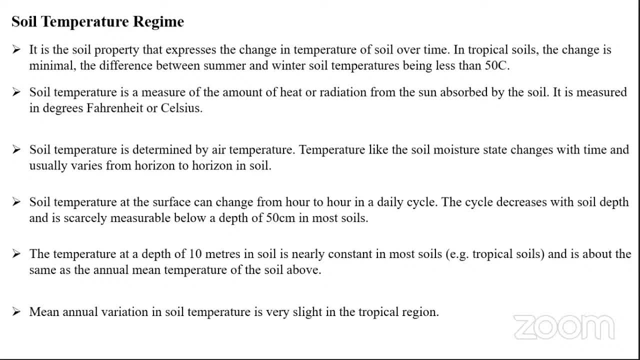 sarcastically measures below the depth of 50 centimeters and naturally the soil temperature- mostly we will. we will see most of this temperature will be seen around the 50 degree celsius. the temperature, the depth of 10 meters are nearly constant in most of the soils, so naturally up. 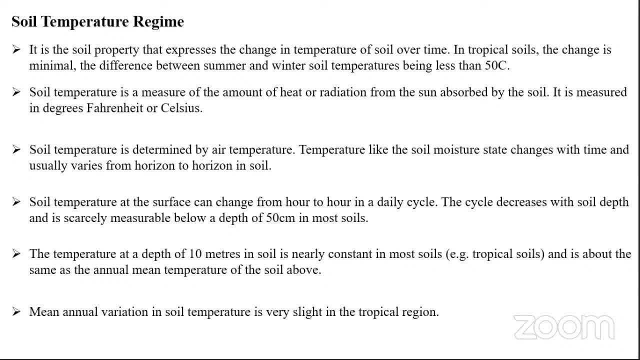 to 10 centimeters, 10 meters, sorry, 10 meters- the temperature will be. the another will be same. and about the seams, annual mean temperature of the soils. above and again, if you see that above and we can calculate, and based on that we will calculate the annual meal temperature of the soils, mean annual mean, annual variation soil temperature. 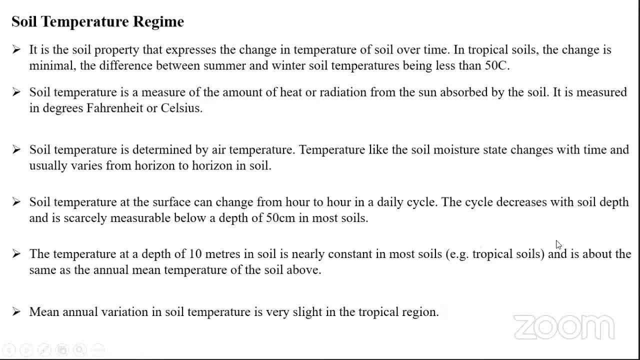 is very slight in tropical regions. so natural students in tropical regions, in tropical soils we can't see much variation. only in other climatic conditions- semi-arid or even a humid condition- we can say the major difference in the soil temperature, because precipitation plays a role in temperature. so these are the students. this is what i want to say. please note down this table. 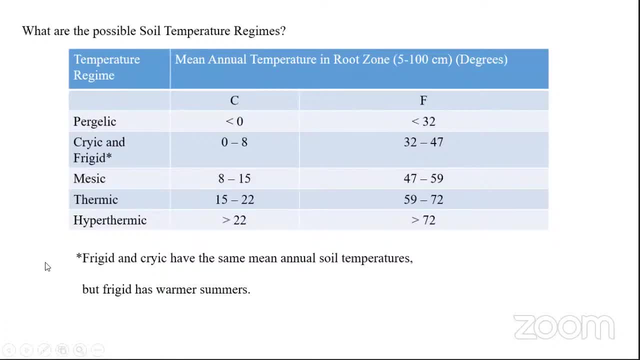 in this table itself. you will get hardly. at least you will get one, one question from this table. please note down this. so what are the different, different types of soil? the temperature regimes are there rigidly in, say, if i want to say in a sentence, i say centigrades, it is less than zero. 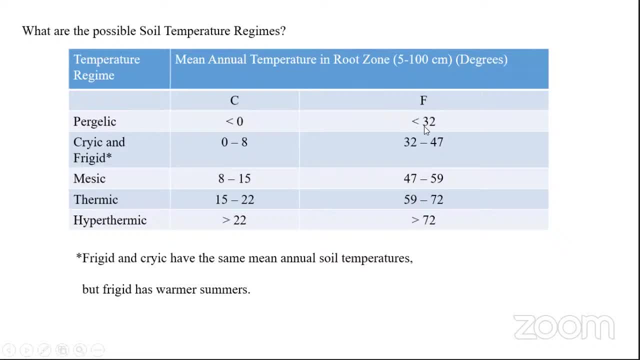 resilient means in fahrenheit, if you want to say. in fahrenheit means it is less than 32 degrees. that is the degree farm heat, and again it's kike or frigid. uh, both have a minimum annual temperature. these two have both the same mineral mean annual temperature. 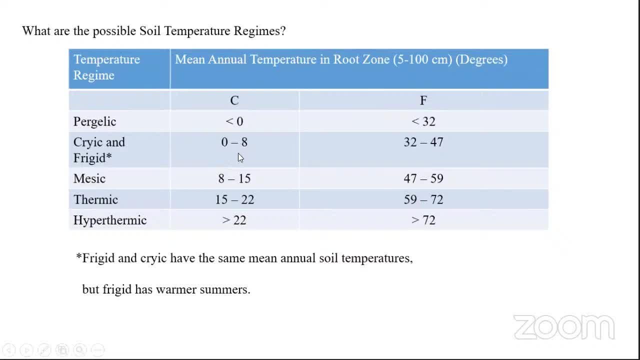 you can see the strike, or frigid, we can say around 0 to 8 degree celsius. if you want to say in a farm, heats that 32 to 47 day, uh, fahrenheit, cells, fahrenheit and the music which is music. another one is intermittent, which is around 8 to 15 degree celsius, whereas if you want to say in fahrenheit, 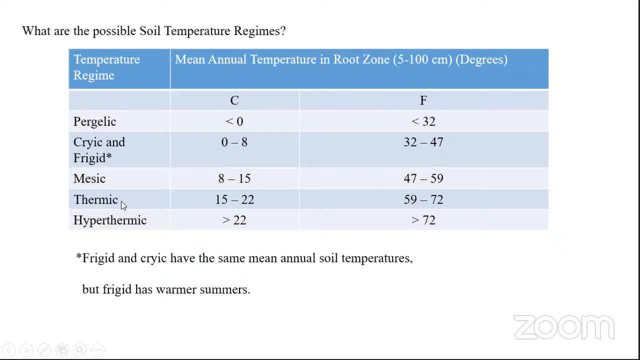 47 to 59 fahrenheit thermic. thermic means hot, you can. thermal heat you can, you can. just to remember the, the, they just make it like that, like that sense. there it may be 15 to 22 degrees celsius. the farm heat means, if you want to conversion, around the 59 to 72 day. 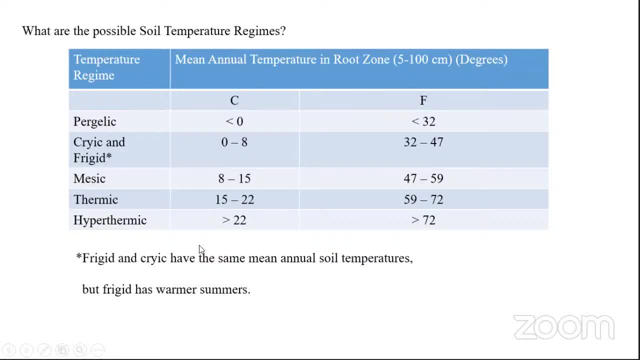 72 farm heats hyperthermic students. hyper, hyper, very high. hyper means very high. what do you say? this is more than 22 degrees celsius. if you want to send, fahrenheit is more than 72 degrees celsius. students, regarding with indian conditions: in india mostly you will see only celsius degrees. 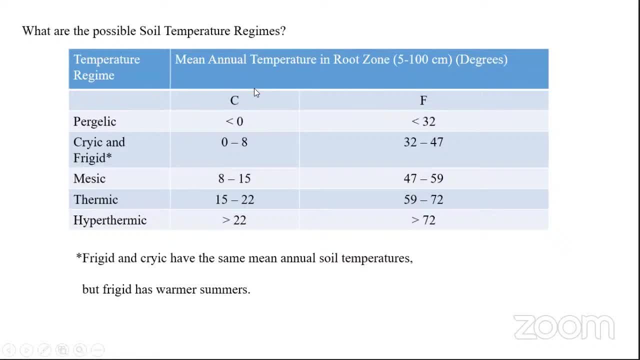 this is very important. most of our questions will come from celsius degrees but, safe side, if you are interested in learning more, you can refer to this one where we mentioned all these very more important things. but remember this one also so rigidly: or frigid music, thermic and hyperthermic. 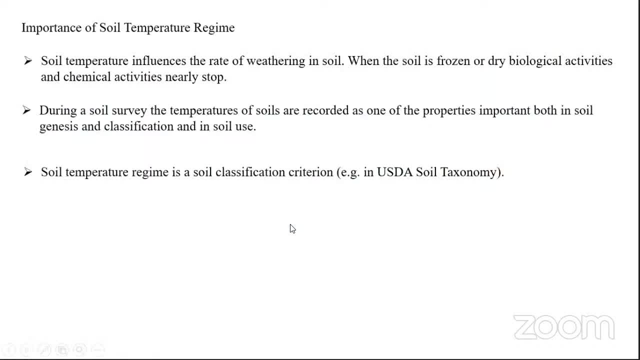 these are the important in overall. this is overall, this lecture. this is very important thing we have to see next. so what is importance of soil moisture and soil temperature regimes? what is the important thing? so soil temperature influence, the rate of weathering in soil. naturally, temperature place a. 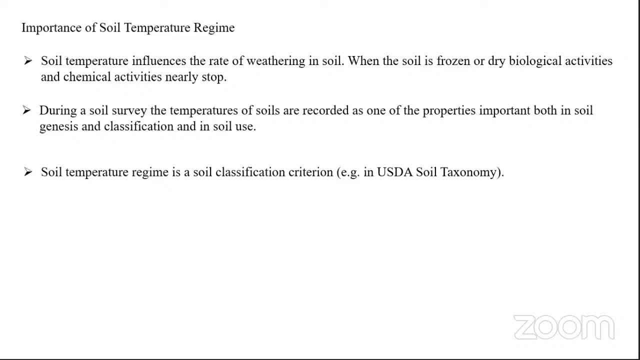 biological activity and chemical activity nearly stops. that's what we say now. actually, if you see these, uh, monarch beards, uh, some beer, some one particular animals will be there. if the season comes, what will? even frogs will go to the hibernation. because when, when, the, when, the 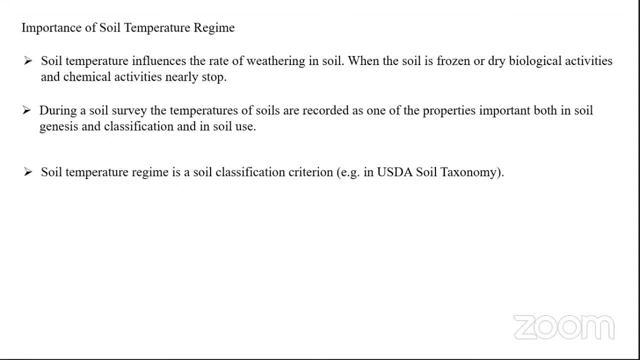 climate is very cold, they will go into sleeping stage because there is temperatures are very less, so natural. the temperature plays a major role in biological activities in the soil and also chemical activities also inside. during a soil survey, the temperature of soil records as an important property both in soil genesis and classification. just similar to the soil. 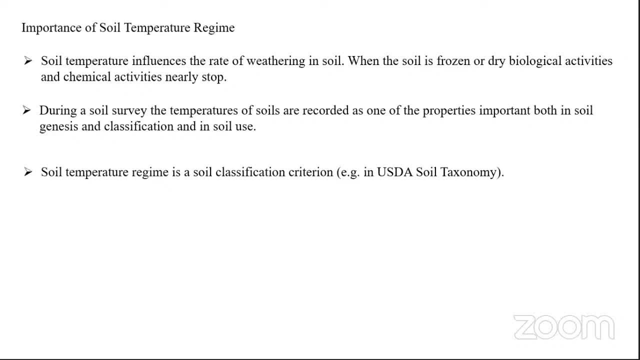 moisture, both in soil moisture regime, also students. if any pedologists want to identify the particular area soil means, he will definitely will focus on these factors: soil moisture regime, soil temperatures. we will see the conditions of the climatic condition and he will compare all the all the climatic situation, relief, topography. what kind of parent material is there? and 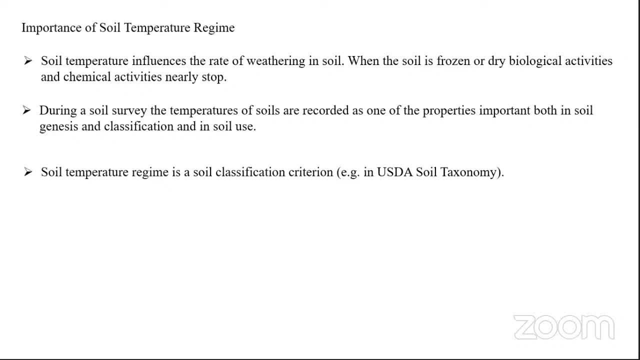 finally, he will come to one conclusion: this particular soil has this type of soil, moisture, resume, this type of temperature is there. this type of parent metal is the relief, is this in this much degree is there? and finally, he will give one notation in, in in his form, this particular area. 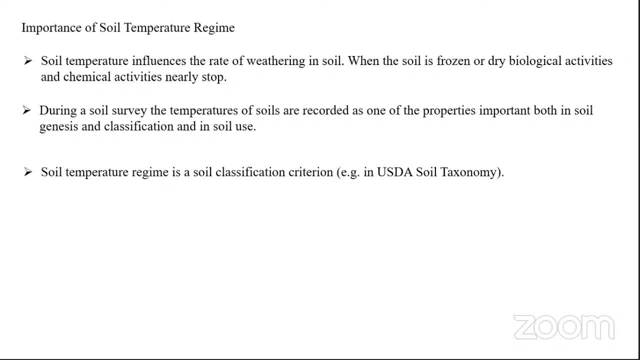 soils comes under this particular order. so this soil here, this company in this particular, so in this particular area, there is a enough, there is a lot of uh soils- are the alluvial soils are there? or aerate soils are there, like that? he will give so soil temper temperature regime and salt cutting. 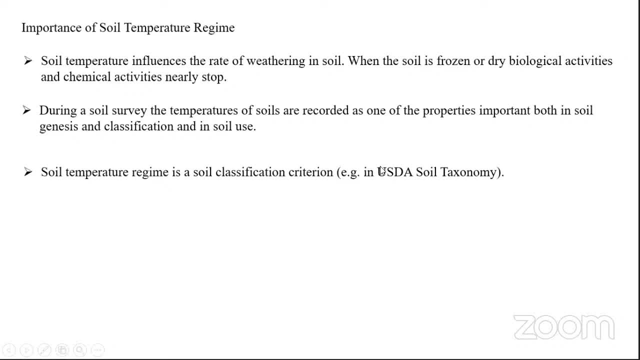 mostly USD taxonomy classification. i will teach these students. i will tell one day they were definitely we will read this again. i think not this week. next week we will read about this usd soil taxonomy- very important and very interesting topic in science. you will see this thing in coming next. 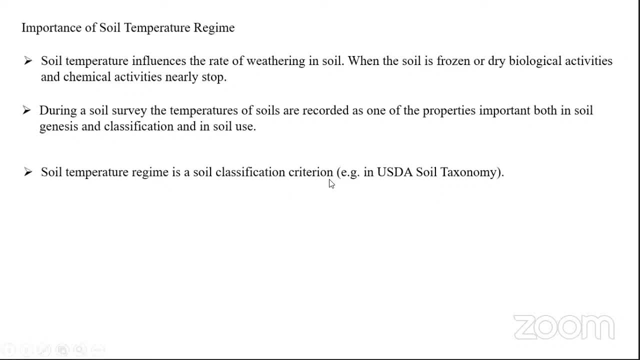 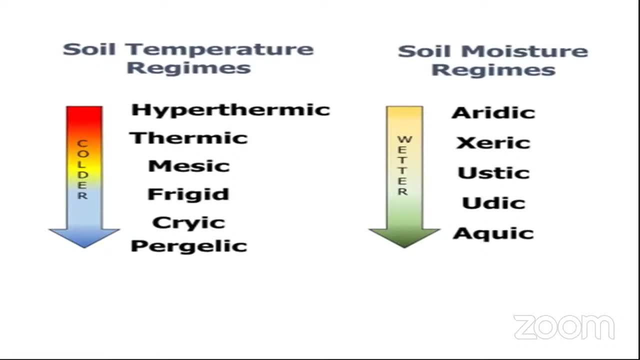 week. so, regarding this today's lecture, that's all, students. a very small lecture. i won't take very lengthy lectures. okay, students, this is what please note. just comparison, for your comparison. this soil moisture, this soil temperature resistance, if i come to down and down, what will happen? the 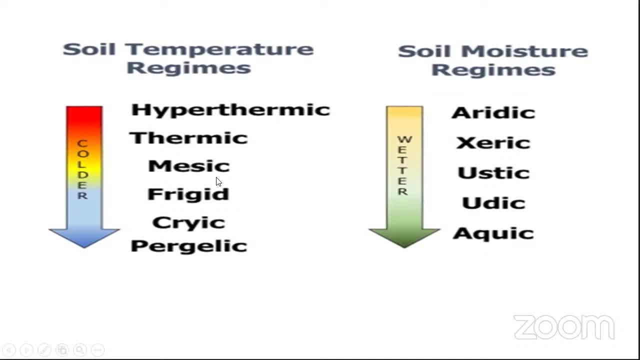 temperature will be reduced. hypothermic is very hot. thermic is very hot. music is very hot. rigid is very somewhat somewhat cool. music is intermediate. rigid is somewhat cool. cry is somewhat a bridge leak is immediately very cool. let's come into the moisture. this is already i. 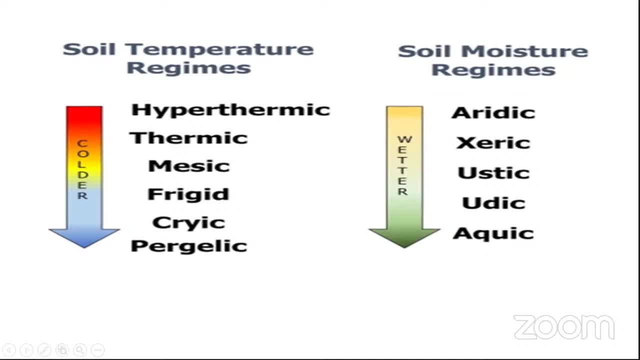 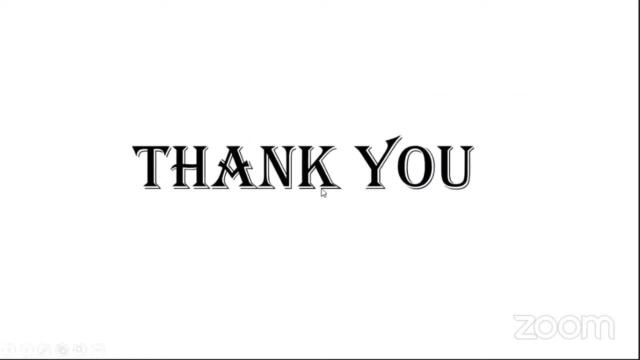 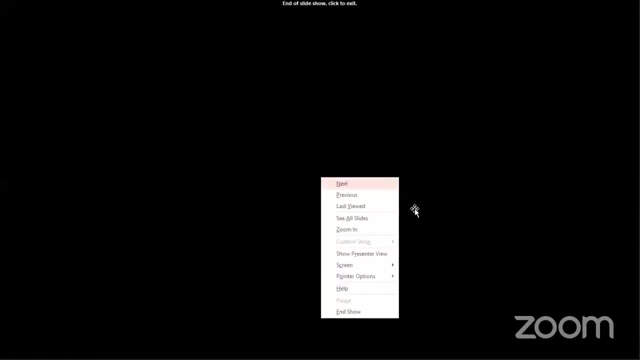 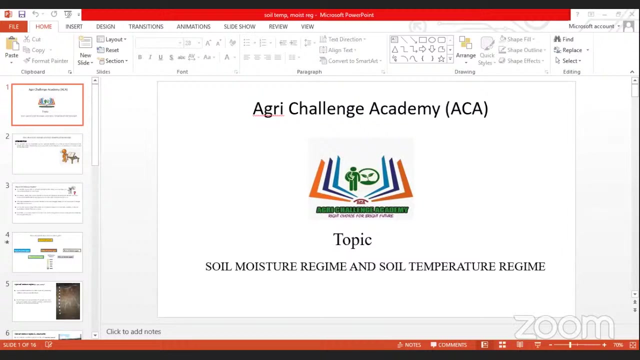 have shown in the previous erratic zergistic. so this is the important slide regarding with soil moisture and soil temperature regime, students. so that's all for today to your students. thank you, very small lecture. you have any doubts? i'm here to clarify any questions, students. oh sorry. 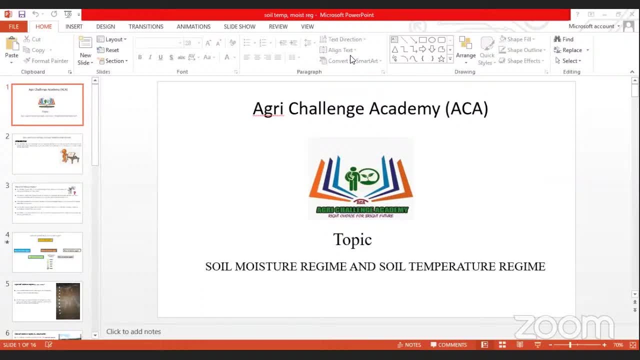 any questions students. look, students, my lectures will be very small and very limited. maybe next class will be some hour. by the way, uh, coming friday, we are planning to uh conduct one exam regarding whatever the lectures we have completed in soil science. so there will be one exam on the soil science the 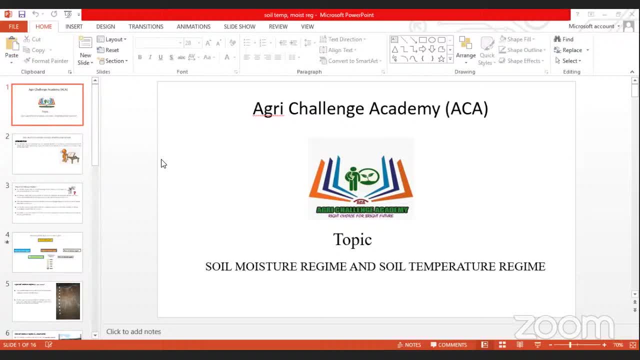 lectures which, whatever we complete, is on, i think, in fertility, we have completed few lectures. in pedology, i have completed, uh, more than three or four lectures i have completed. so by compiling all this, we will go for one test. so please test your knowledge, so prepare well. questions will be very fundamental. 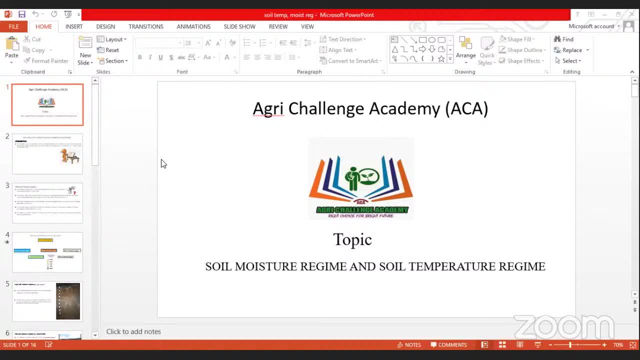 there will be one or two. there will be applied questions. that is for your test, your capacity of knowledge. okay, any questions. also, any questions, no, no, okay, i think. hey, students, uh, i think today lecture is very small and very limited, but you read students once, read it before you read some. 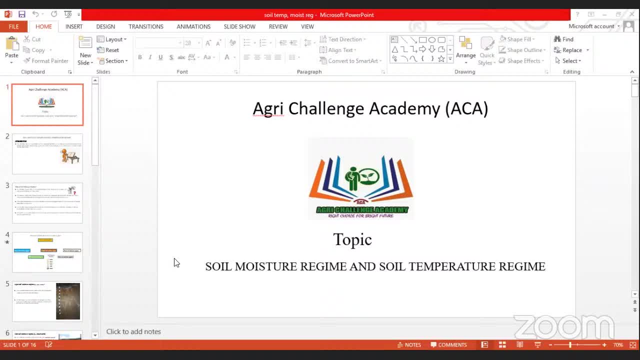 you may know, you are in the literature department. some ah you may not have in today before going: textbook of pedology: there is nothing. finally, is there any questions? one student said no and rest. all. I will clear. okay means okay, no means no, okay, can I leave them? can I leave? yes, sir, okay, okay, okay, okay. students, I think. 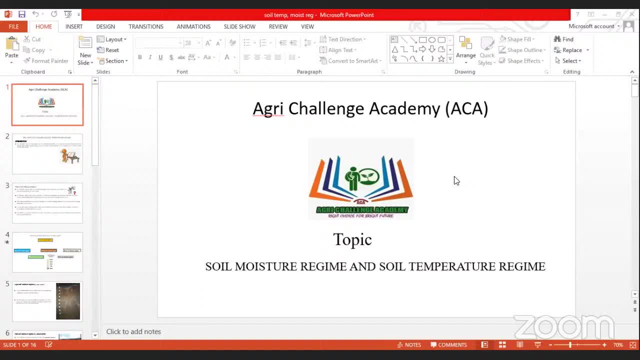 next you have a class at 8 pm. that is English class as well as English class. yes, sir, okay, okay, okay, students, I think next you have a class at 8 pm. that is English class as well. actually saw yesterday, he faces some technical problems.